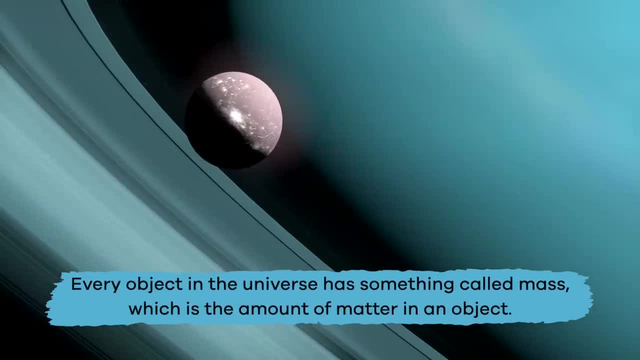 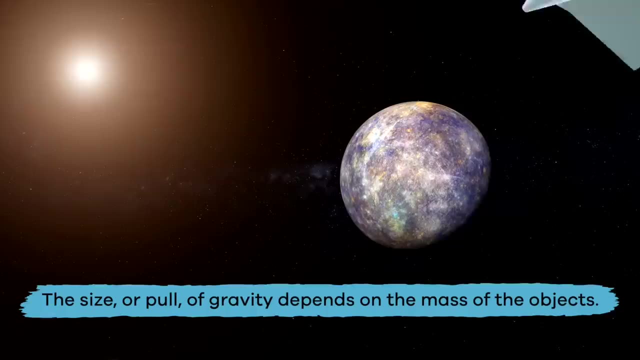 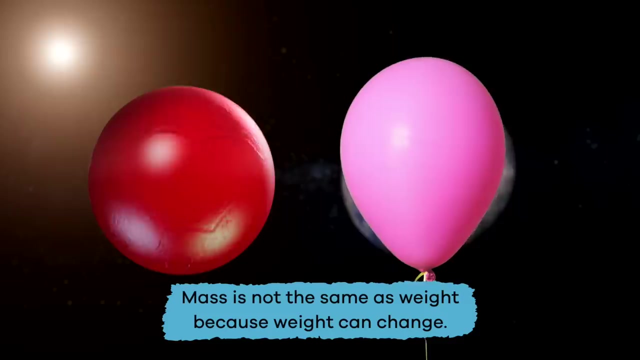 float off into space. Every object in the universe has something called mass, which is the amount of matter in an object. The size or pull of gravity depends on the mass of the objects. Mass is not the same as weight, because weight can change Mass. 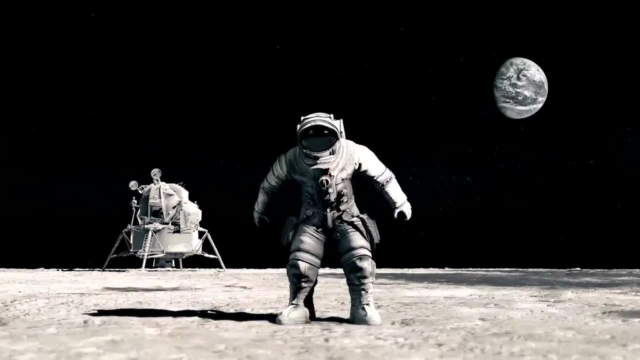 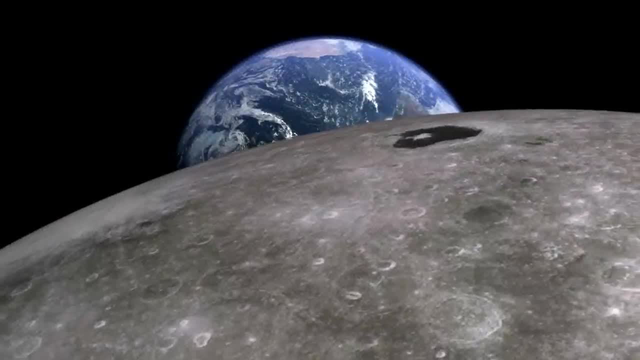 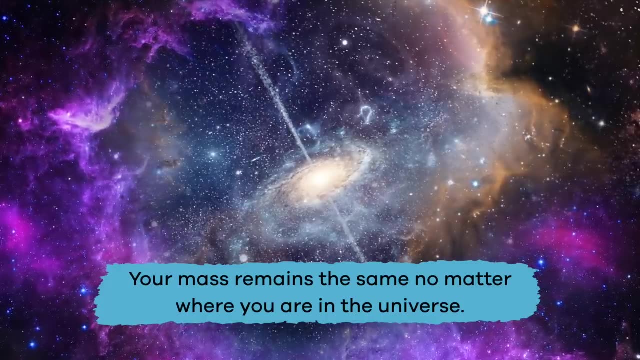 never changes. For example, your weight on the moon is different than your weight on earth because the gravitational pull of the moon is different than the earth's, But your weight remains the same, no matter where you are in the universe. Here's an interesting 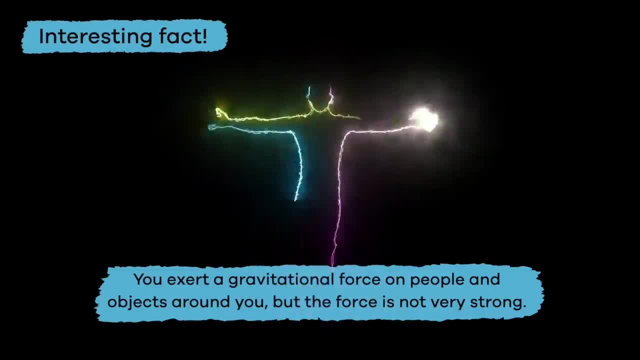 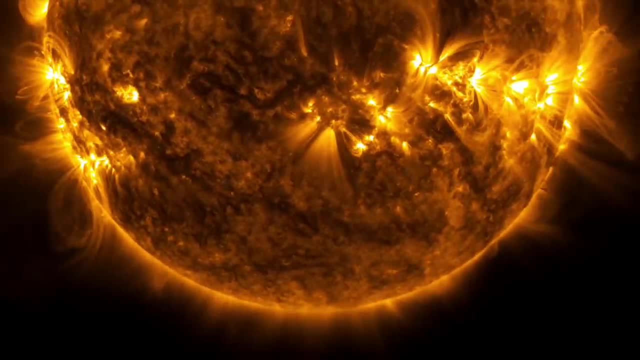 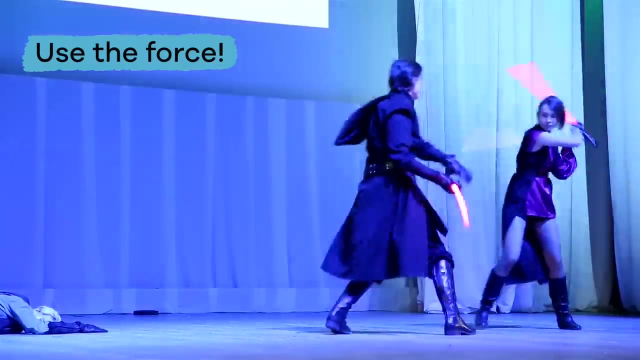 fact, You exert a gravitational force on people and objects around you, But the force is not very strong. This is because you are not as massive as the sun, earth or moon. But the next time somebody tells you to use the force, you can say: I already am Because you are. 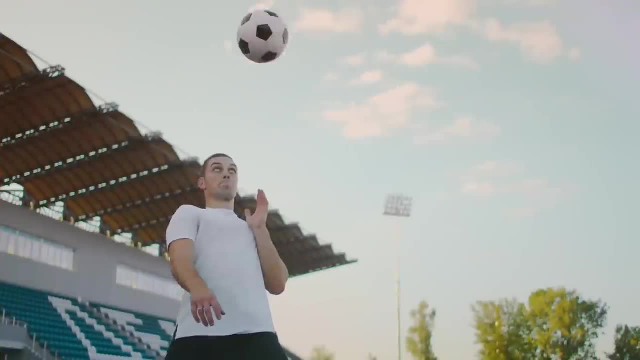 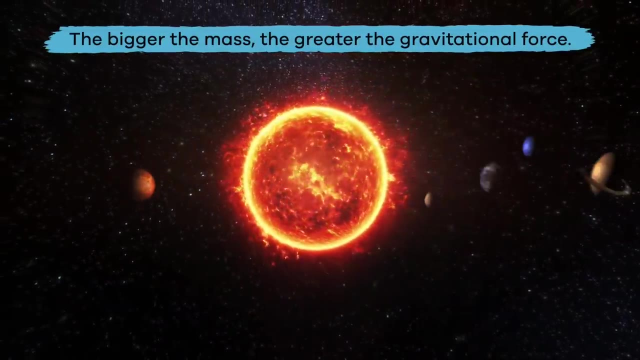 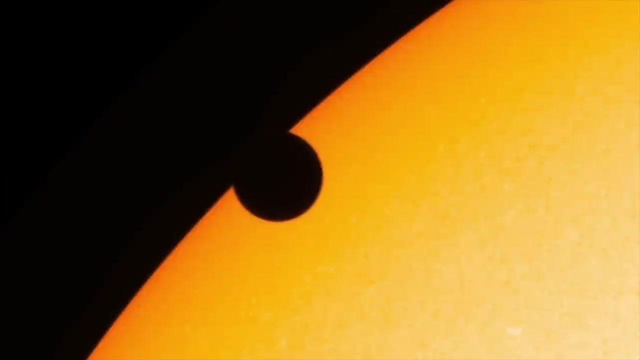 experiencing and exerting gravitational force all the time. Remember this: The bigger the mass, the greater the gravitational force. This is why all of the planets in our solar system revolve around the sun. The sun is so large compared to the planets that each 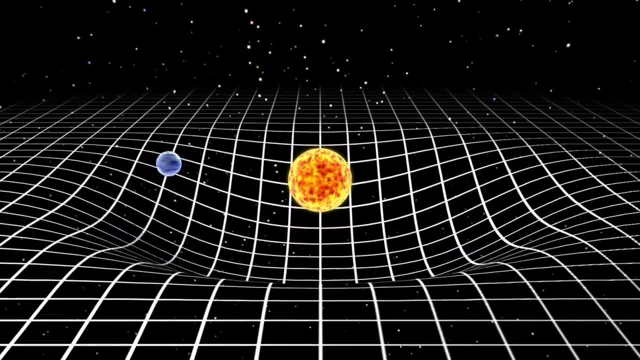 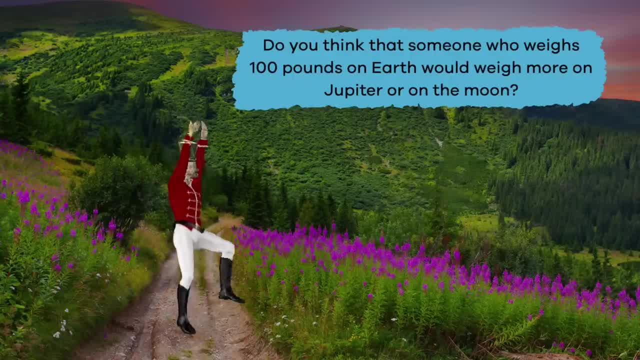 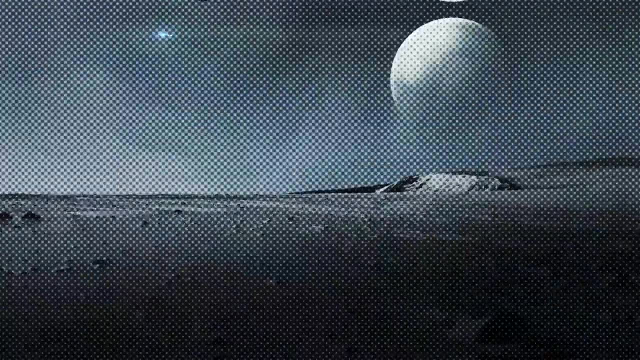 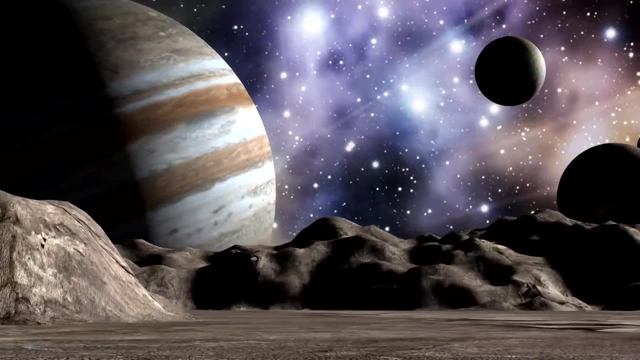 planet is pulled or attracted to the sun as they orbit around it. Let's look at an example. Imagine someone who weighs 100 pounds on earth would weigh more on Jupiter or on the moon? If you said Jupiter, you're right, Since Jupiter has more mass: its gravitational pull. 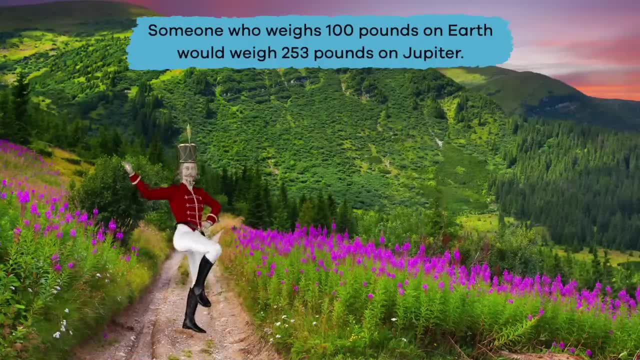 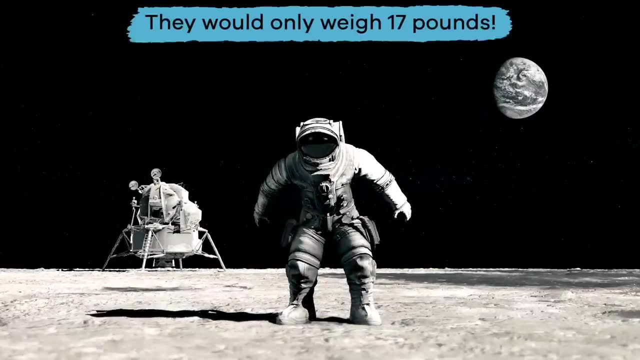 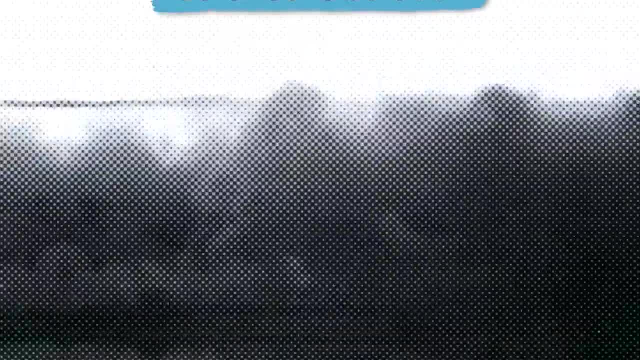 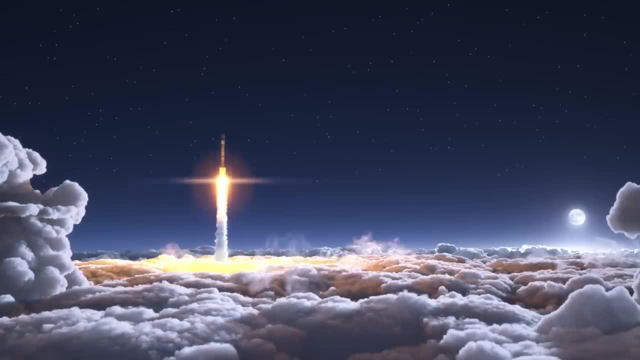 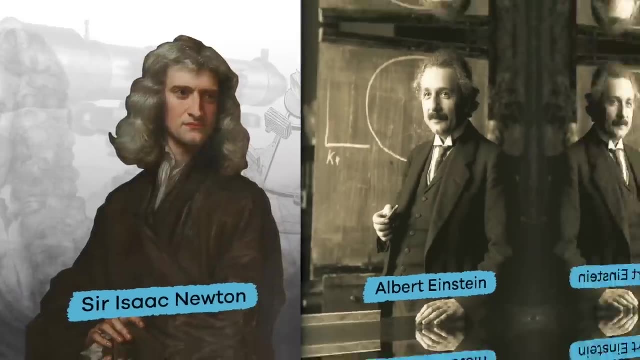 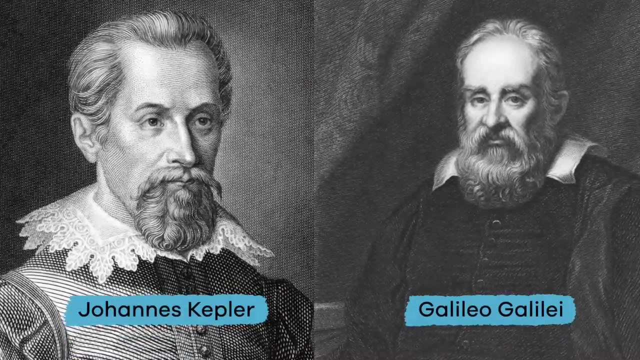 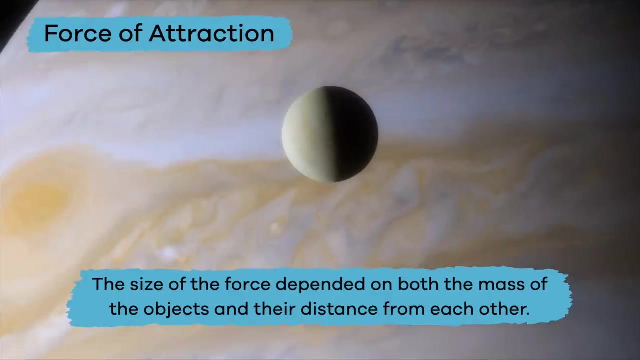 scientists who discovered, researched and experimented with the concept of gravity: Sir Isaac Newton and Albert Einstein. First up is Sir Isaac Newton. He studied the work of other scientists and realized that gravity was a force of attraction and that the size of the force depended on both the mass of the 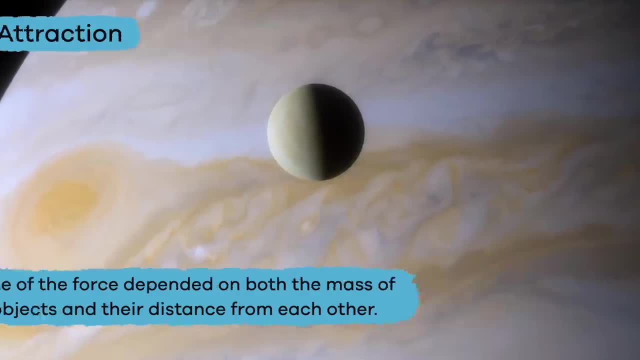 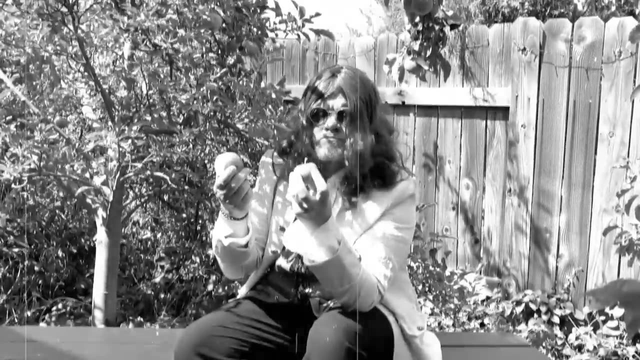 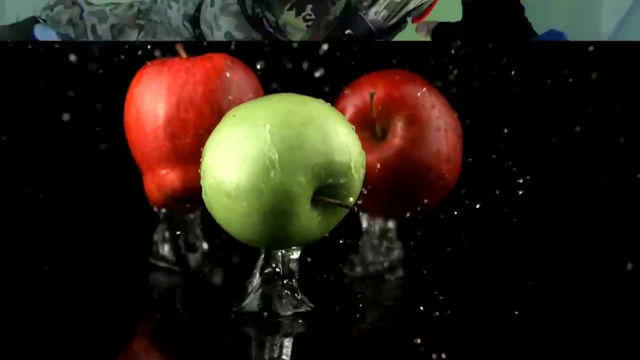 objects and their distance from each other. Sir Isaac Newton is the scientist who watched an apple fall from a tree and realized that there was a force at work. Newton wondered why the apple falls straight to the ground and not sideways. He realized that the force that makes objects fall to Earth and the force that 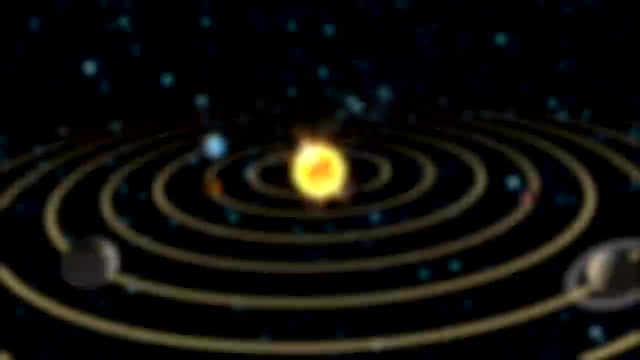 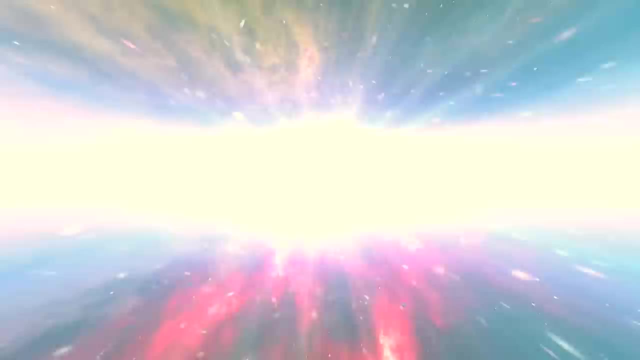 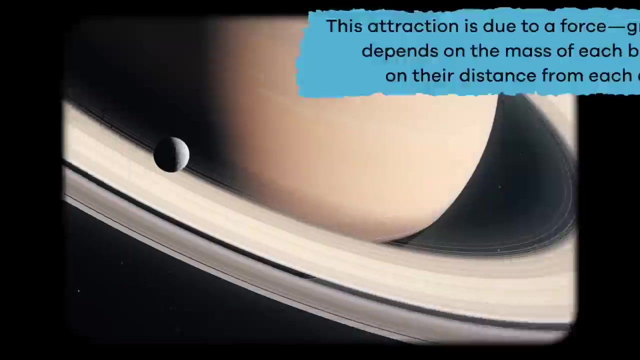 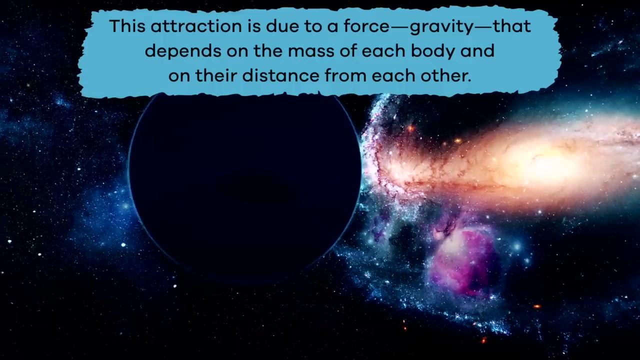 keeps the planet in their orbits are the same force. Newton's law of universal gravitation was published in 1867 and states that every celestial body in the universe attracts every other celestial body. This attraction is due to a force- gravity- that depends on the mass of each body and on their distance from each other. 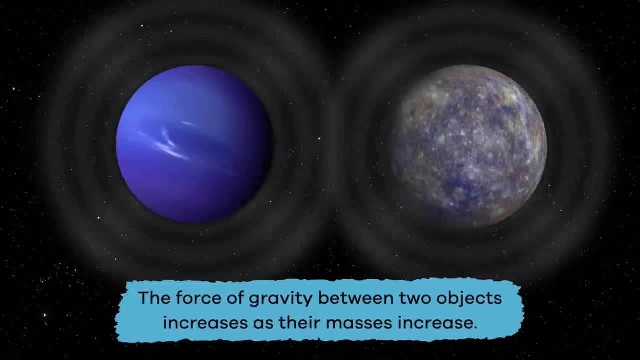 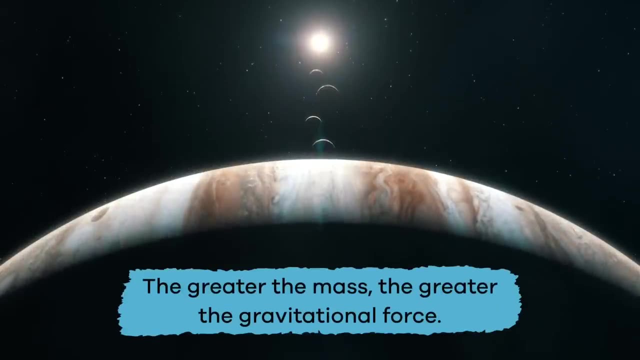 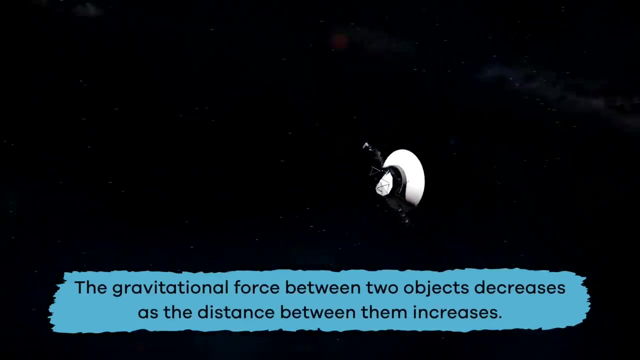 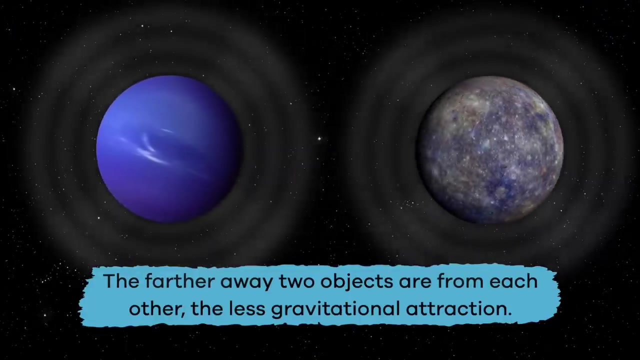 The force of gravity between two objects increases as their masses increase. In other words, the greater the mass, the greater the gravitational force. Also, the gravitational force between two objects decreases as the distance between them increases, which means that the farther away two objects are from each. 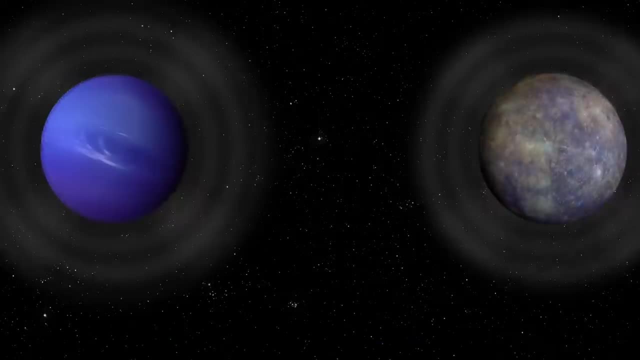 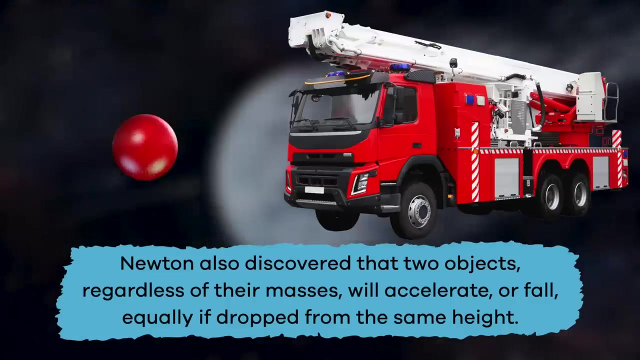 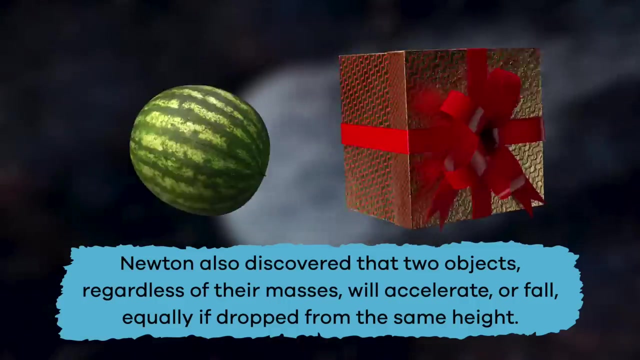 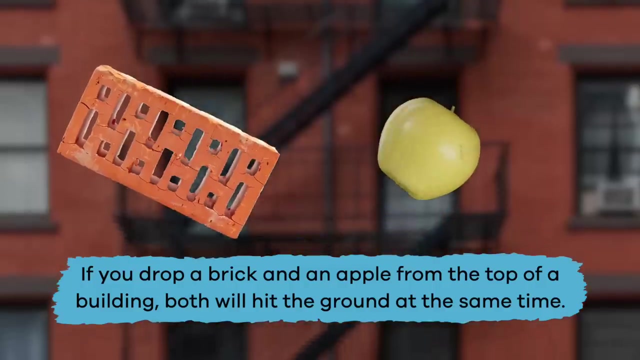 other, the less gravitational attraction. The closer 2 objects are, the greater the attraction. A student also discovered that two objects, regardless of their masses, will accelerate or fall equally if dropped from the same height. For example, if you drop a brick and an apple from the top of a building, both will hit. 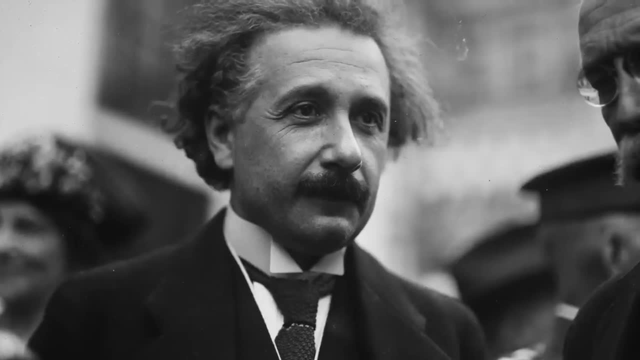 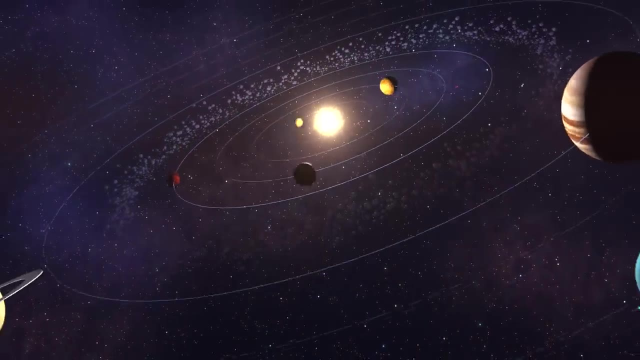 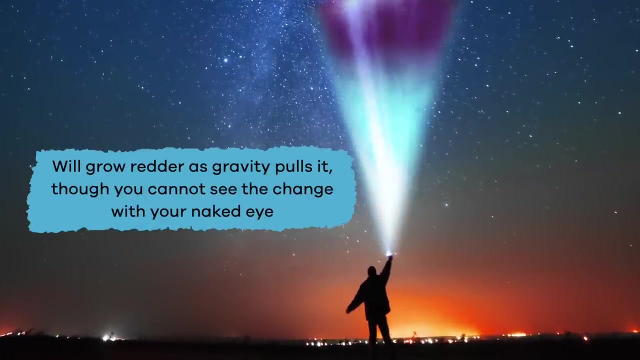 the ground. at the same time, Another famous scientist, Albert Einstein, discovered that gravity not only pulls on mass, like a planet, but also on light. A flashlight shined into the air will grow redder as gravity pulls it, though you cannot. 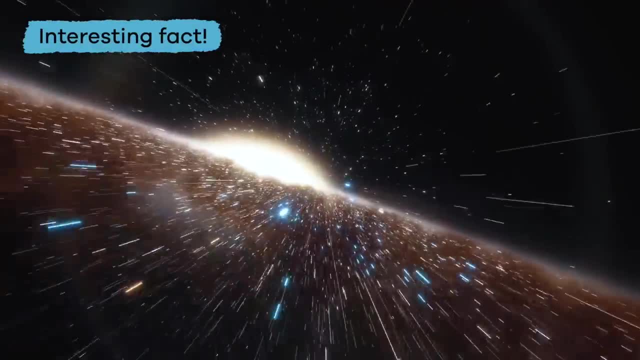 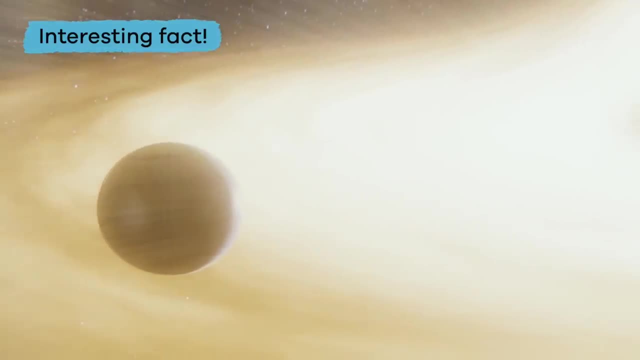 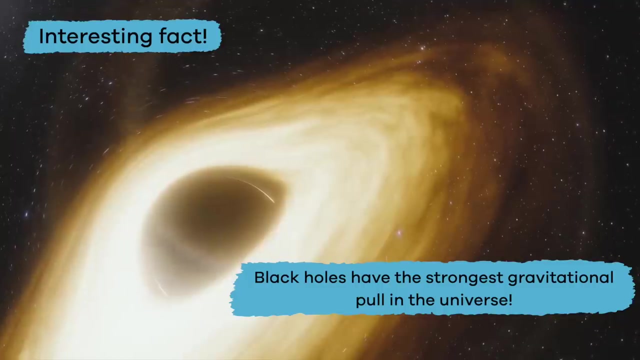 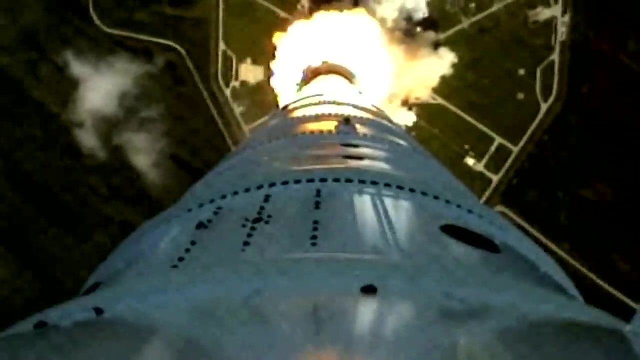 see the change with your naked eye. Here is a final interesting fact. A black hole has so much mass, in such a small volume, that its gravity is strong enough to keep everything from escaping even light. Black holes have the strongest gravitational pull, And scientists have only scratched the surface of studying them. 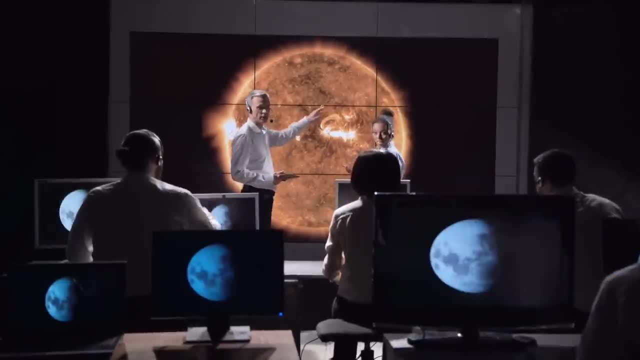 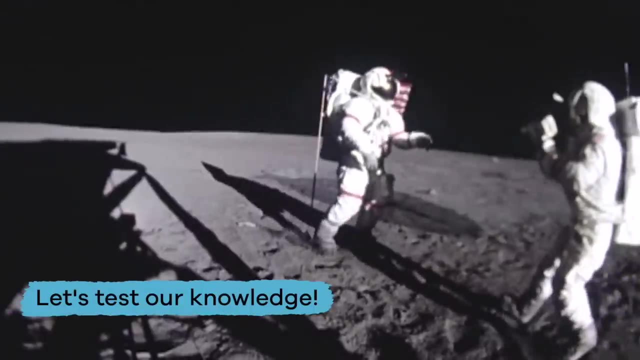 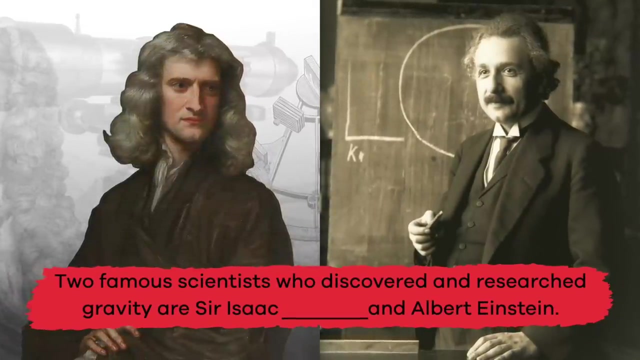 Maybe someday you will be a scientist who discovers even more about gravity. Okay, our brains are full of new and exciting information. Let's test our knowledge. Fill in the blank: Two famous scientists who discovered and researched gravity are Sir Isaac Blank and Albert Einstein. 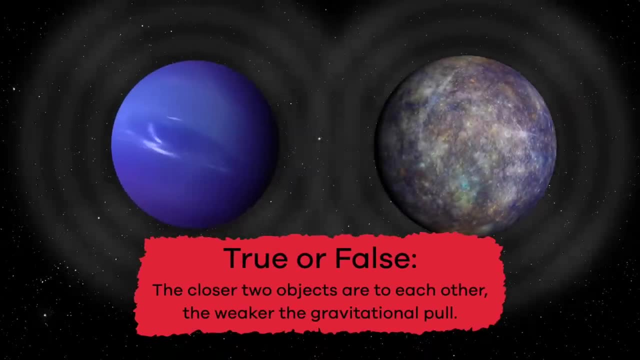 No doubt You are right. Your answers are super smart, That's true. So which ones of you are right? Oh, that's me. I am right. I am from Washington DC. I am up on the moon. Up on the moon. 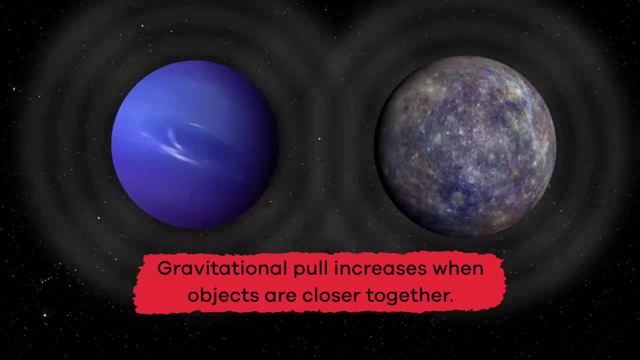 Of course You are right. I have the same answer. I am from the outskirts of Washington DC. I am up on the moon. This is great. We have to be sure. we are right, To be perfectly sure. you are right, it is a given. 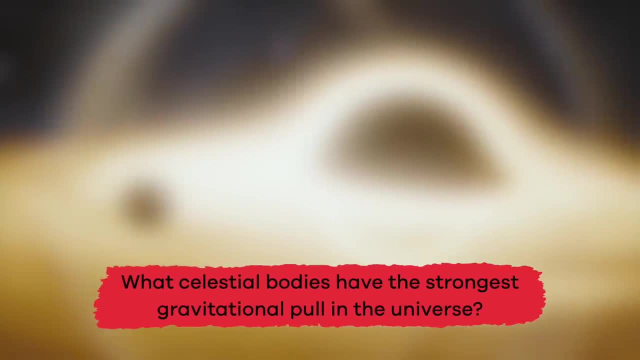 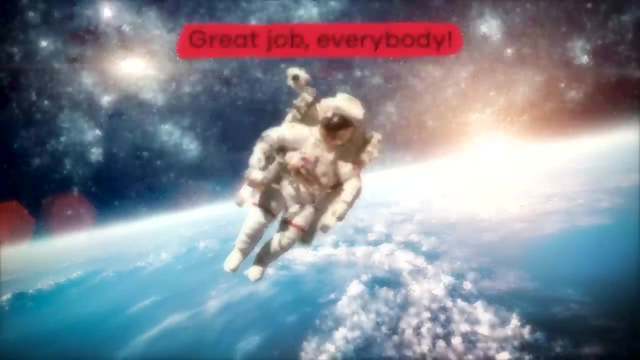 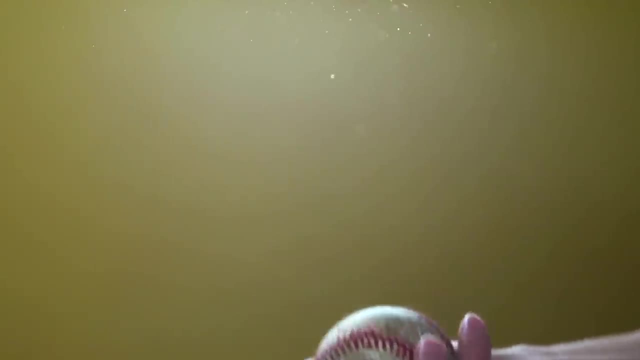 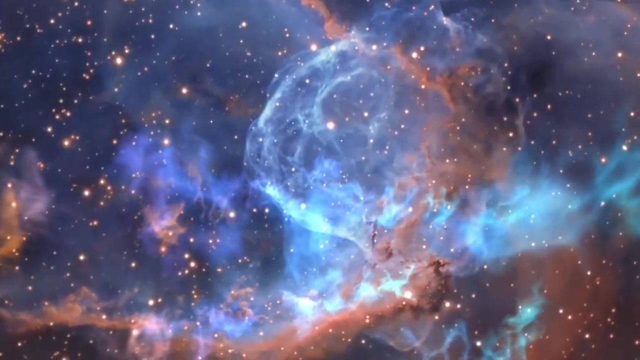 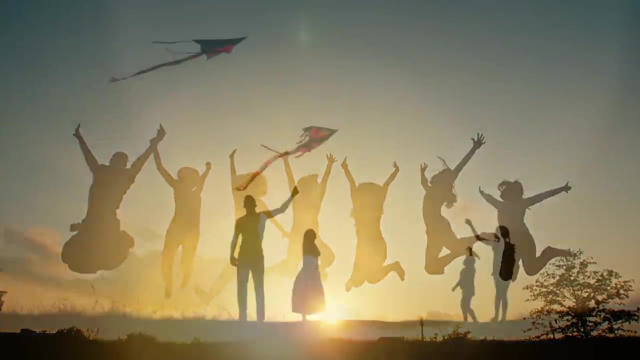 Three stars us. even when we're not aware of it. It literally keeps our feet on the ground and is a vital part of our planet and universe. The next time you see an apple falling from a tree or feel the force of gravity as you jump in the air, remember what you've learned today and share it with your family.